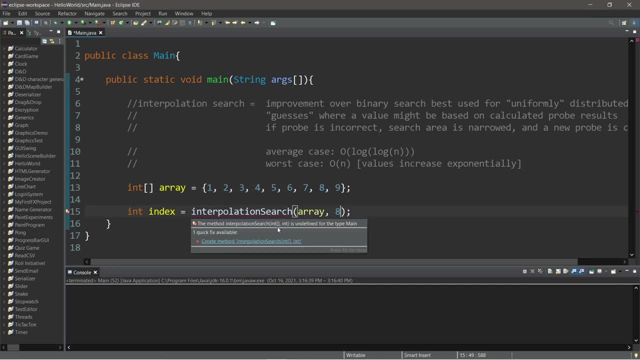 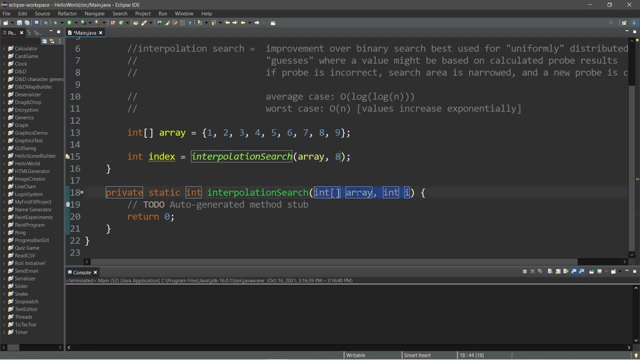 the number, maybe eight? Okay, then let's declare this function Private. static int interpolation search. There are two of them. Let's say that we have a number of eight. Let's say that we have a, two parameters, an array of integers and our value we are searching for. I'm going to rename. 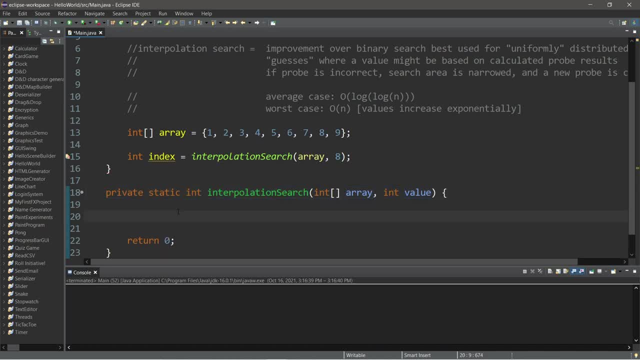 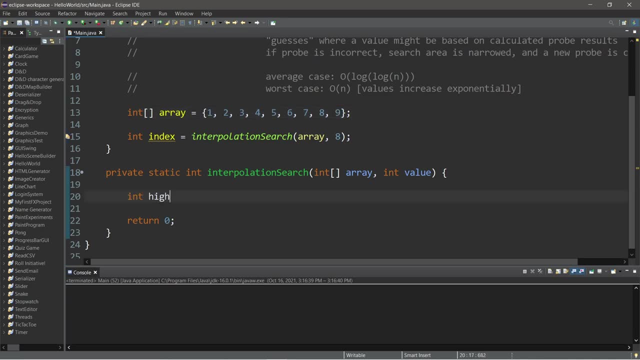 this parameter as value, so it's more descriptive. The first thing that we're going to do is calculate the upper bound and the lower bound of our searchable area. So int high will be the higher bound of our searchable area, and this will be our array's length minus one, And the lower bound is: 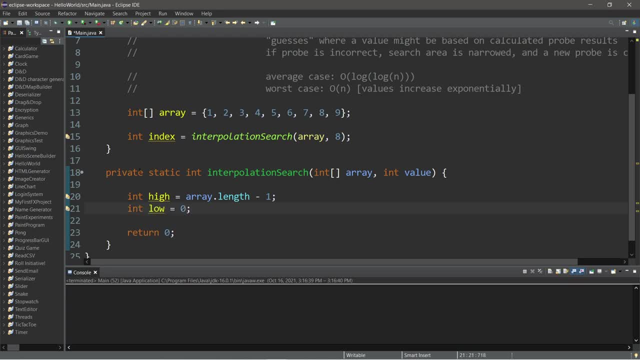 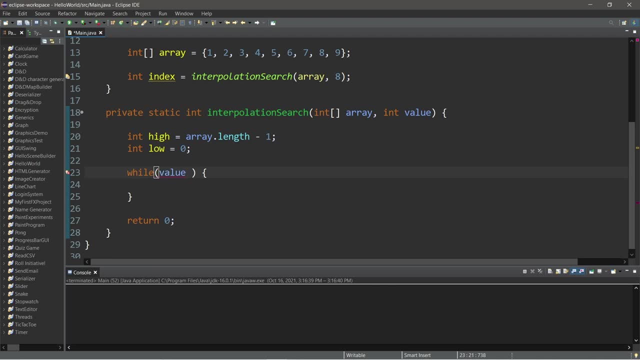 well, the first index, Int low, and I will set this equal to zero. Using a while loop, we will create a new searchable area. The condition within our while loop is: while our value is greater than or equal to our array at index of low, the lower bound, and our value is less than or equal to, 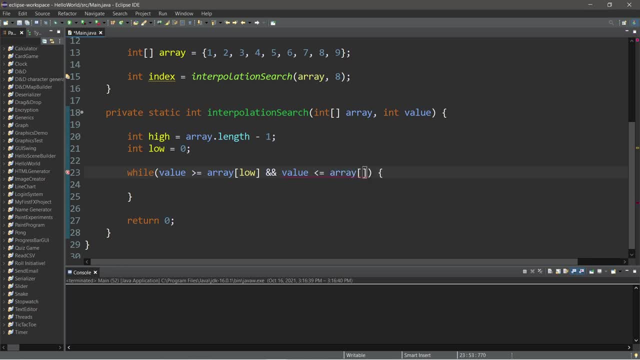 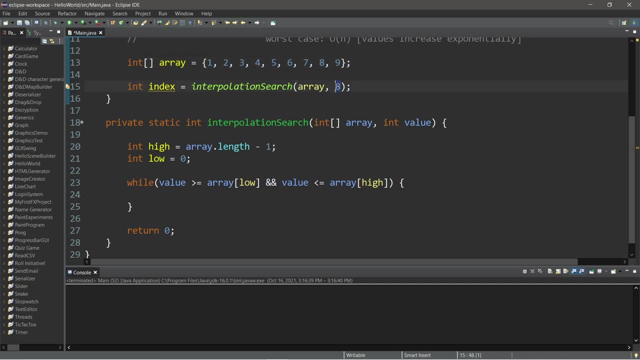 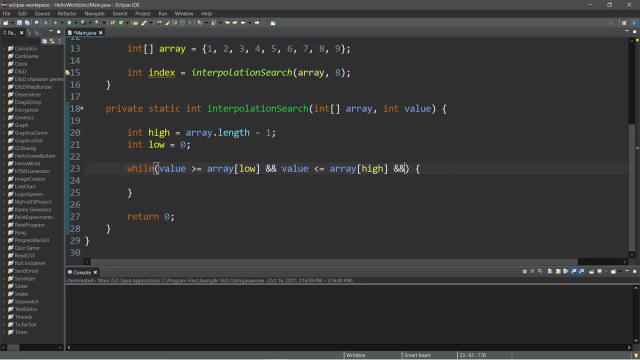 our array at index of higher bound And our sizable search area is going to shrink after each iteration. So while our value is within the new searchable area, keep on probing, keep on searching. I'm going to add another condition too. Int low is less than or equal to high After each iteration. 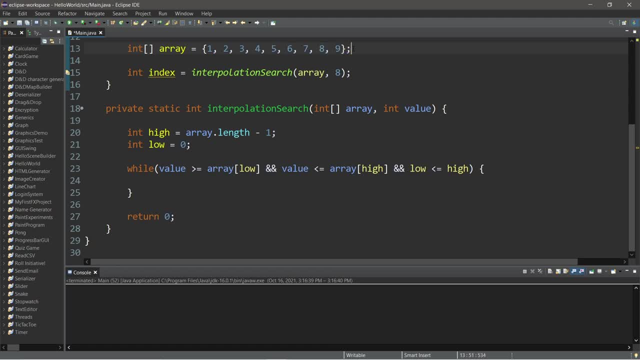 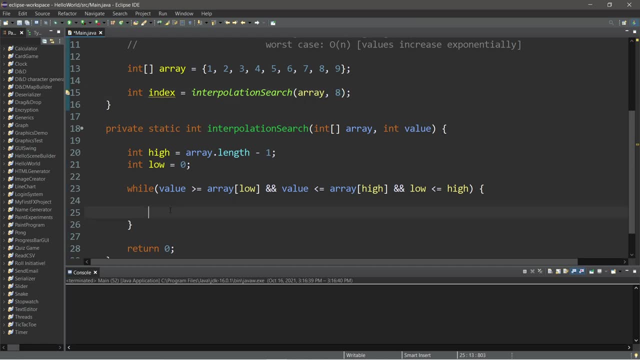 our searchable area is going to shrink. Once our searchable area is zero elements, well, we can't search anymore, so we might as well exit. Now here's the formula to calculate where our value is probably going to be, and our guess will be referred to as our probe Int. probe equals. 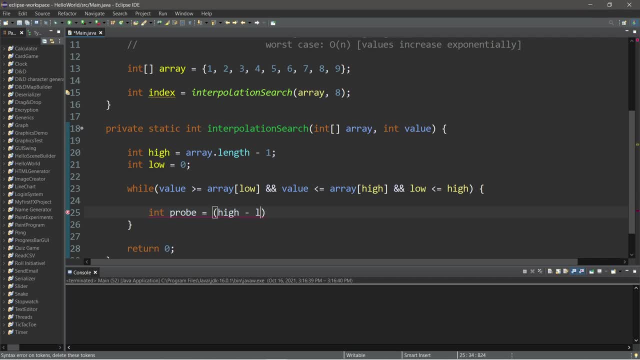 and here's the formula: high, minus, low times our value minus array at index of low, our lower bound divided by array at index of high, minus array at index of low. I'm just going to add low to the front of this and I'm just going. 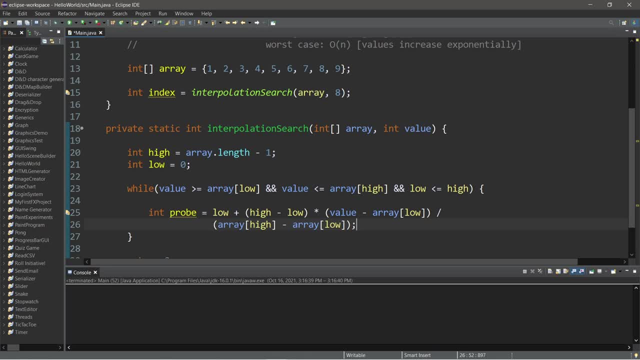 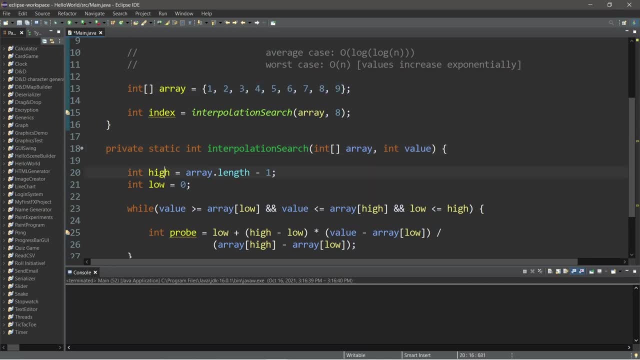 the size of our current searchable area: high minus low. So to begin with we have nine elements times the value we're searching for, minus the value at the lower bound. so eight minus one divided by the value at the higher bound, minus the array at the lower bound. Then, at the end, 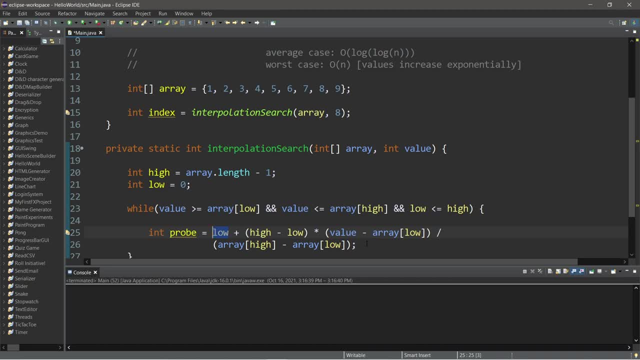 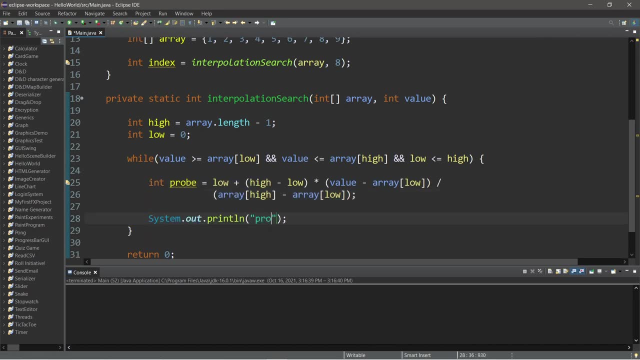 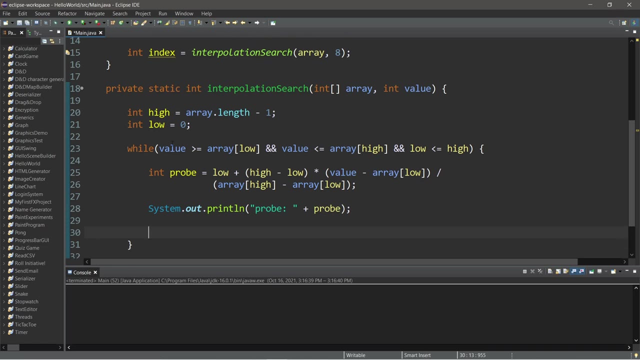 we're just tacking on whatever our lower bound currently is. So it's a complex formula. All you have to do is just copy this. So during each iteration I'm going to display our probe. This is going to be essentially our guess, And let's check to see if our probe is equal to our. 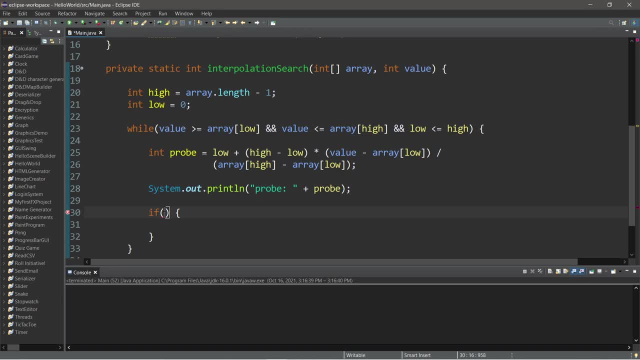 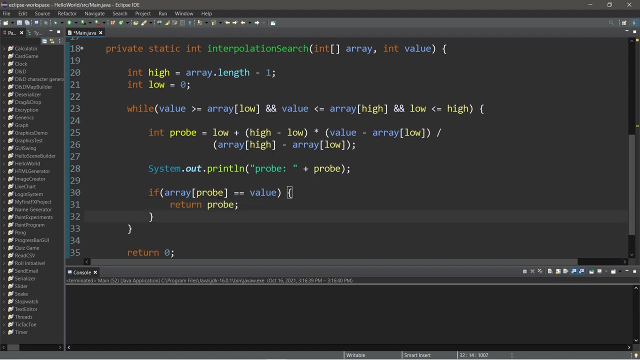 value. So, using an if statement, let's check to see if array at index of probe is equal to our value that we're searching for. If it is, let's return our probe. This is the correct index. Else, if our guess our probe is incorrect, we'll need to narrow down our search area. So, using an 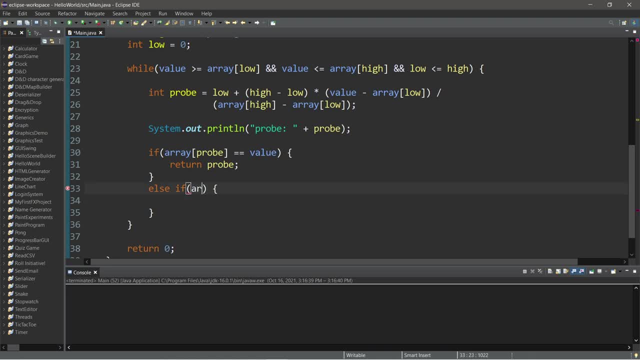 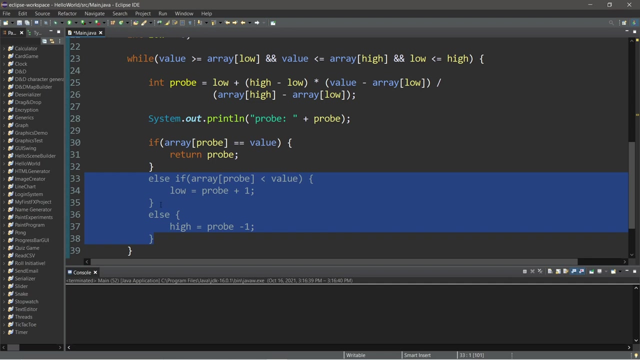 else if statement, let's check to see if array at index of probe is less than our value. If that's the case, we will need to set the new lower bound: low equals probe plus one, Else high equals probe minus one. Now here's the deal with these statements. We're currently searching for the 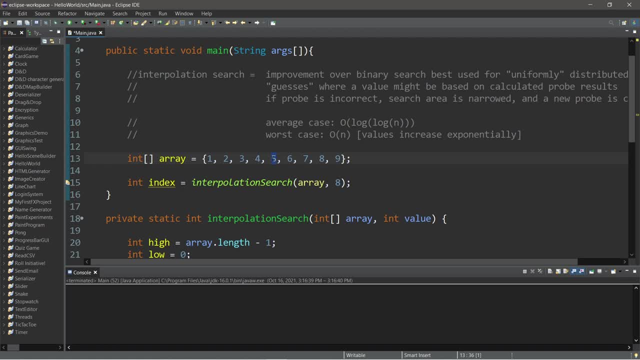 number eight. If we guess our probe is at, let's say, five and our value is greater than this probe, we can disregard this portion of the searchable area. So we're moving the new lower limit, the new lower bound, to just after where our probe was. 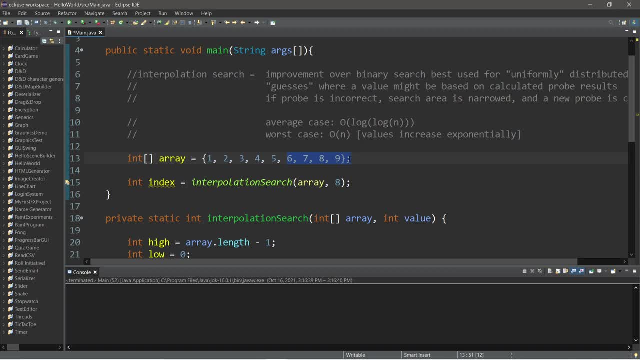 six. So this is the new searchable area, And then we'll calculate a new probe based on this data. If we're looking for, let's say, two and our probe says it's likely here at five, well then, since two is less than our probe, we can disregard all of this data, and this would be our new. 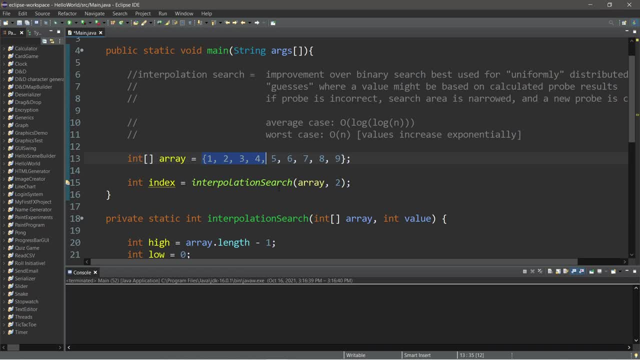 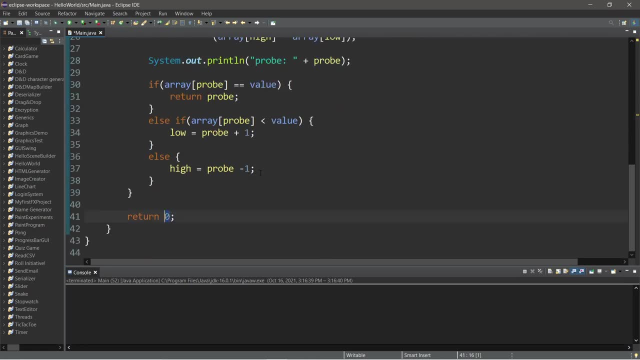 searchable area, We would move the higher bound of our data down to just below our probe. So that's kind of the idea. So at the end, if we do not find our value, let's return negative one as a sentinel value. So back within our main function, let's check to see if the value returned. 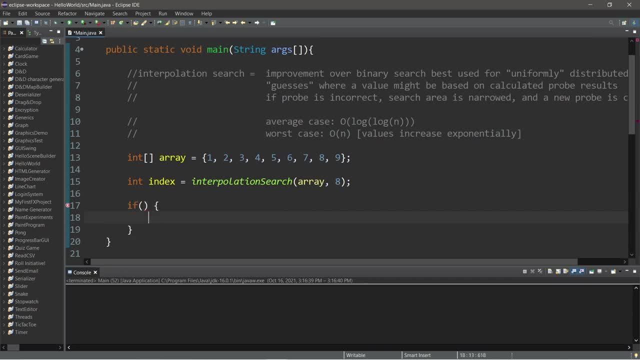 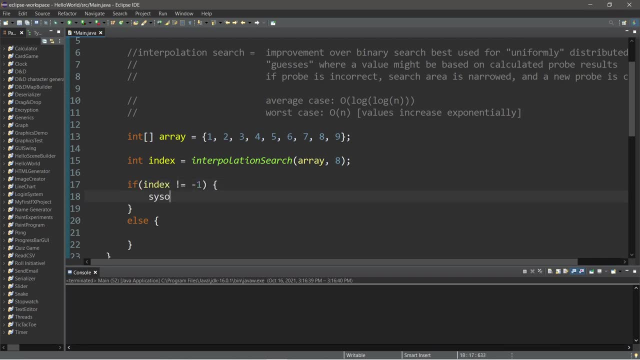 does not equal negative one, Using if else statements: if index does not equal negative one, then let's print a message: Systemoutprintln- Element found at index plus index. Else- element not found. Okay, so this should work. Let's run it. 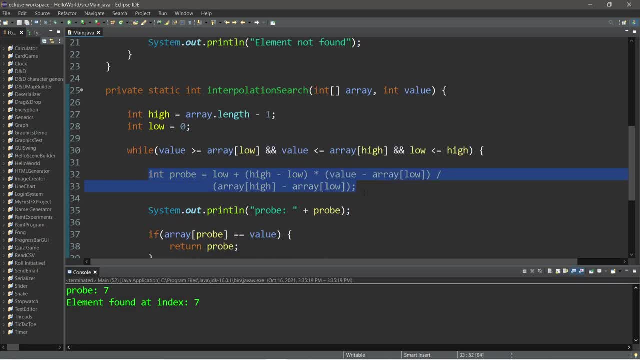 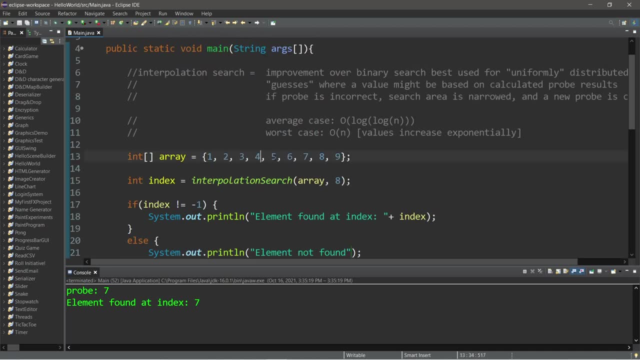 So we are searching for eight. So this formula calculated that this value is likely at probe seven, index seven, zero one, two, three, four, five, six, seven. And this was the first iteration of our wild loop We were able to find: 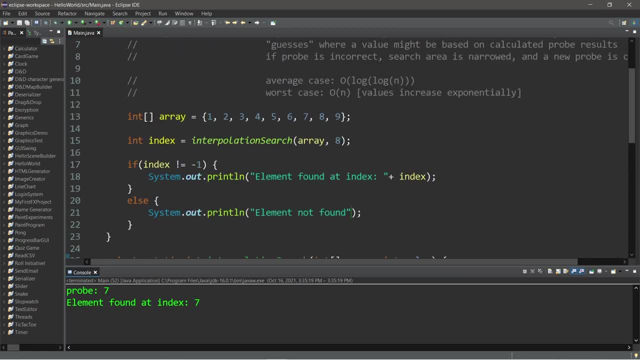 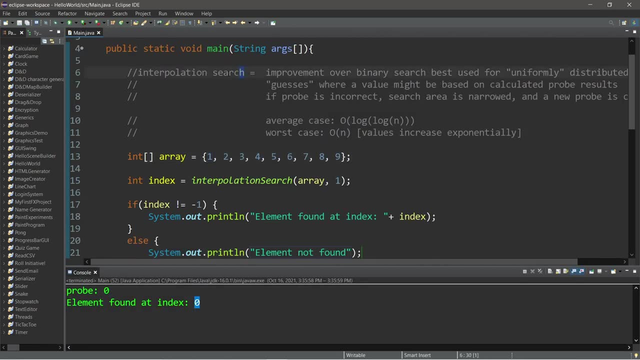 our value eight on the first iteration. So let's find a different value. How about one Element found at index zero? That's the first element. So interpolation searches work very well with uniformly distributed data. These numbers are all increasing by one, So this is a little too easy for our interpolation search. 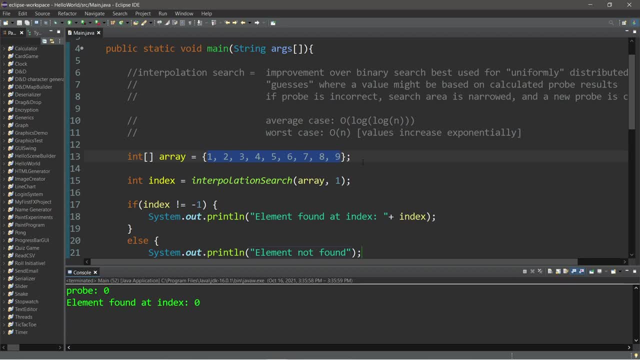 It's guessing the likely index on the first try. So let's create a more difficult data set. So with our new data set, let's say that we will start with one and then double the number of the previous element. So one, two, four, eight, sixteen, thirty-two, sixty-four, one-twenty-eight, two-fifty-six, five-hundred-twelve and one-thousand-twenty-four. 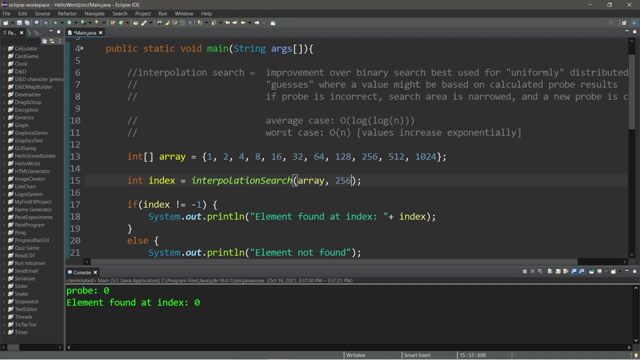 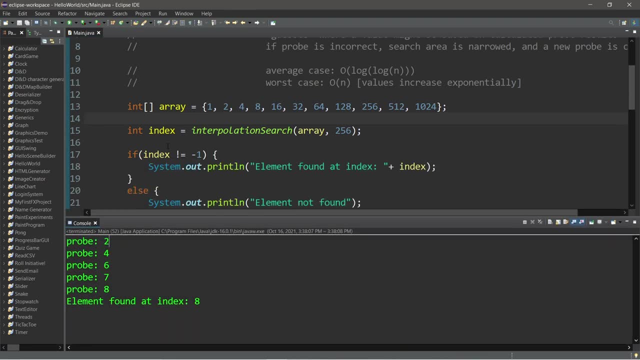 And let's search for the number. what about two-fifty-six? Let's see how many probes this is going to take. Alright, so here's the results. We iterated our wild loop five times. We had five different guesses. After the first guess, this was not correct. 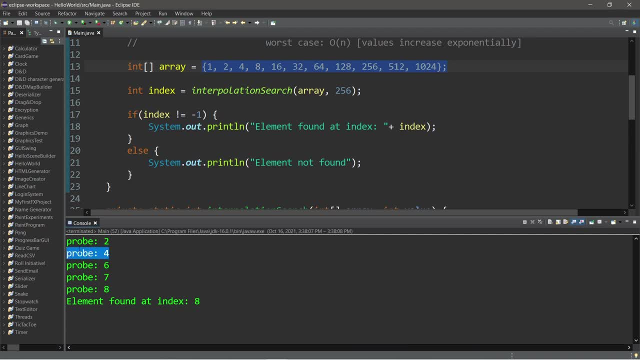 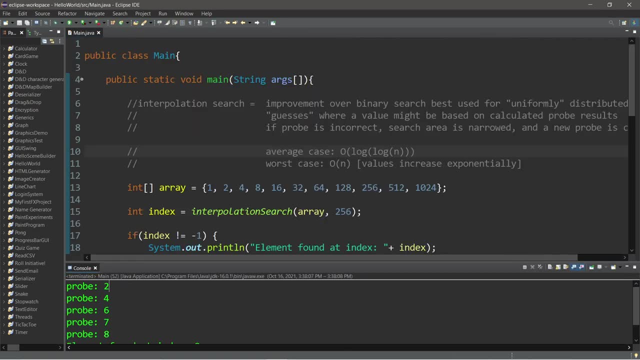 So we narrowed down our search area, then we probed again. This still wasn't the correct answer, So we probed again, and again, and again until we got the right value. So that's an interpolation search. It's an improvement over a binary search that is best used for uniformly distributed data. 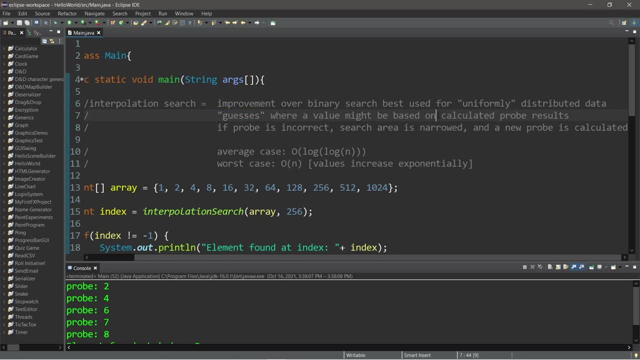 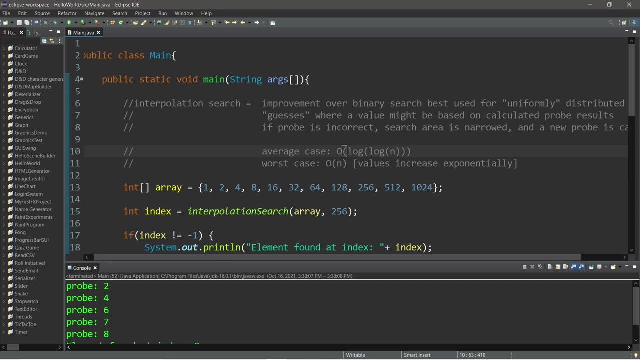 It guesses where a value might be based on a calculated probe result. If the probe is incorrect, the search area is narrowed and a new probe is calculated. The interpolation search has an average runtime complexity of O and a worst-case runtime complexity of O.